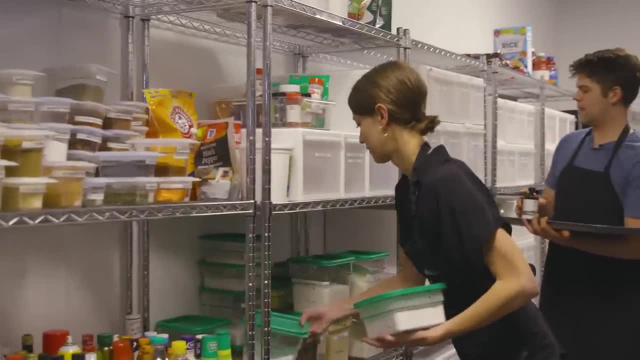 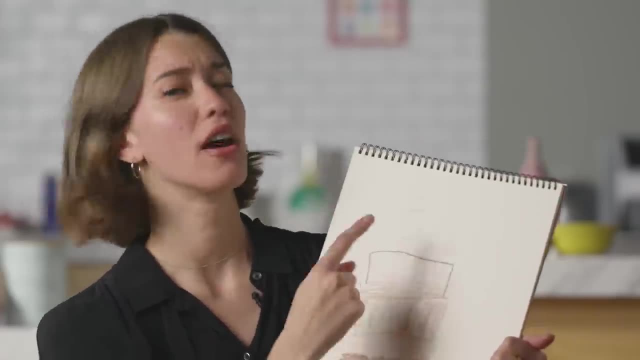 We've got cookie on the bottom: glaze cupcake- half, more glaze cookie, frosting cupcake- half and more frosting. Am I feeling confident? I think I'll get there. I'm going to first make a really nice. 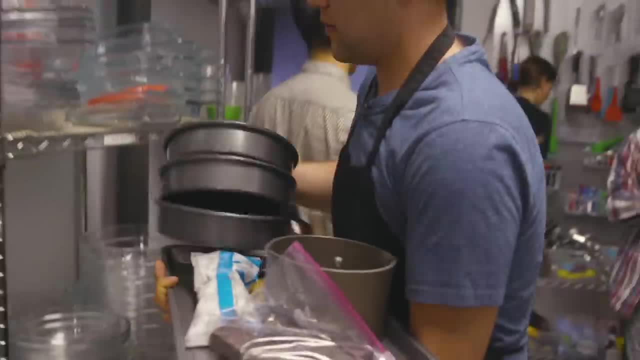 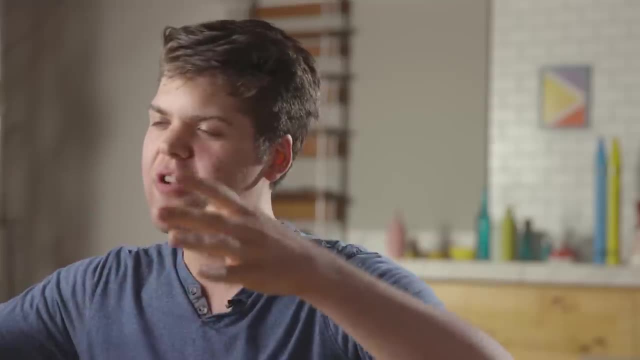 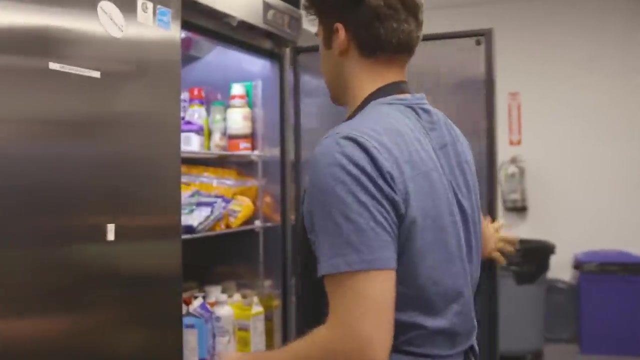 round chocolate cake. then have some great strawberry buttercream frosting, then a giant chocolate cookie with white chocolate chips. more frosting, another layer of chocolate cake. I'll put frosting with a lot of great garnishes like fresh strawberries. Matthew is an amazing cook. He does really great work. He's gonna be a good competitor. 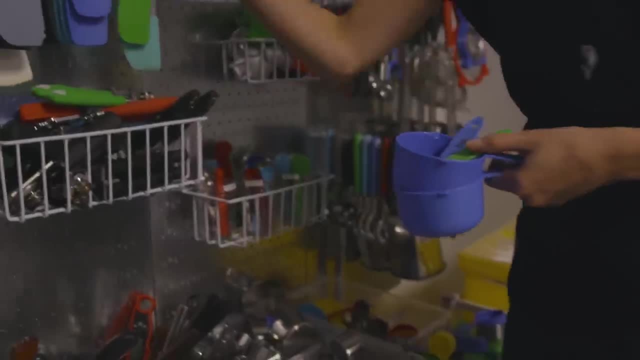 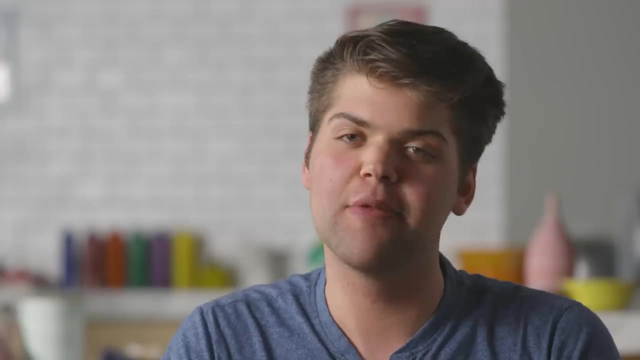 I'm gonna make a really moist chocolate cake, put some strawberry glaze on it, a cookie that fits perfectly on top- frosting strawberries cake and then repeat. Alexis will do her best. I know I'm gonna do my best, but I hope I come out on top. 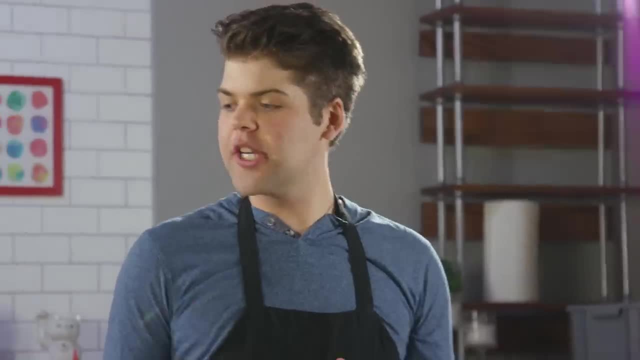 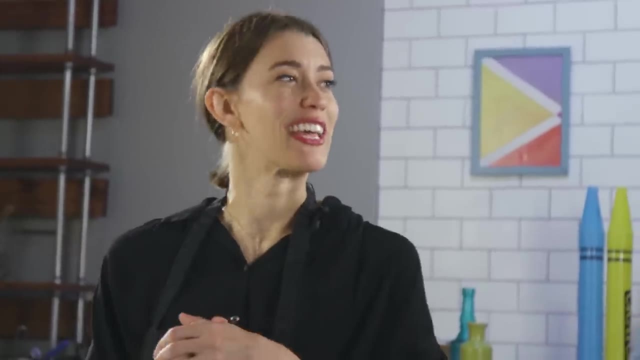 I'm starting with my chocolate white chocolate chip cookies and then gonna move on to the cupcake that I'm turning into just a normal chocolate cake. I too am starting with my cookies and then making like a mini six-inch cake. I just sifted my two flours. 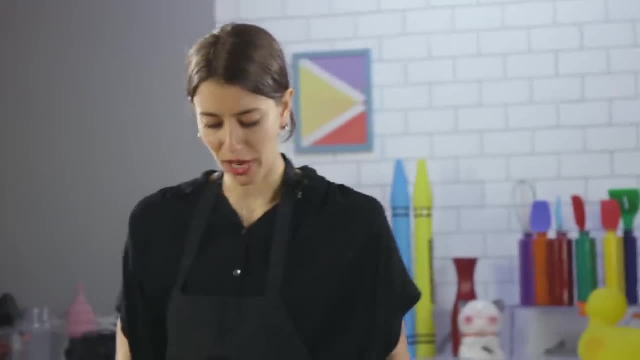 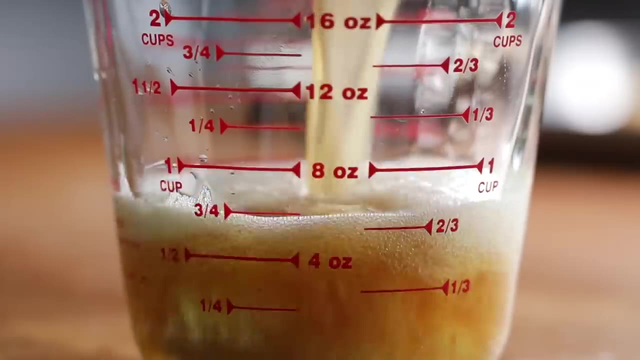 I'm using regular flour and bread flour So I'm gonna brown the butter so it's gonna get this like really dark nutty color. It'll boil down a bit, since some of the fat cooks off, So I just added a bit of water to bring it back up to a cup. Now I'm gonna add the sugars. 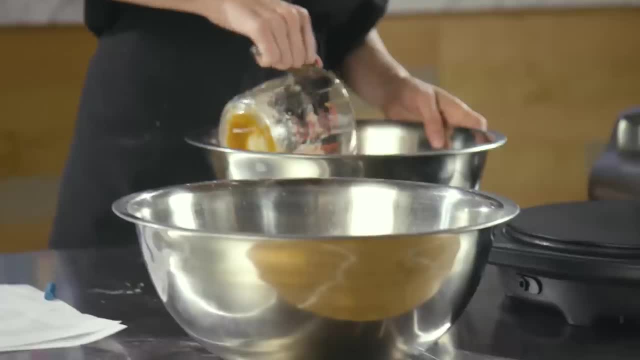 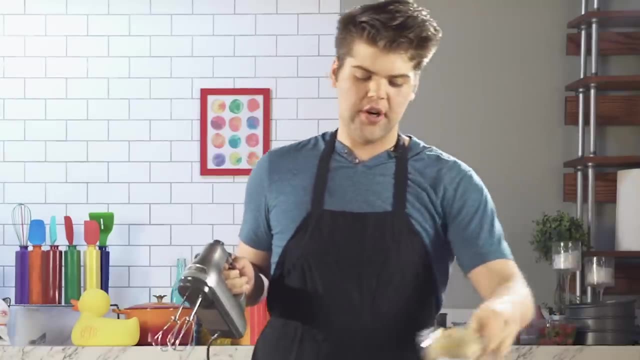 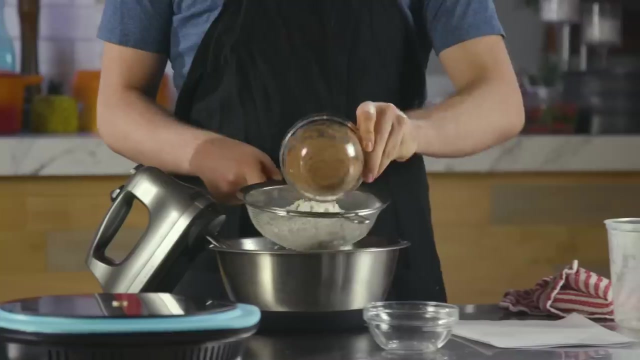 So adding brown sugar, white sugar, and then we're gonna add the brown butter. My god, that looks amazing. So right now I'm starting with the butter, brown sugar and regular white sugar to cream together for my cookies, And now I'm adding the eggs, flour, cocoa powder, baking soda. 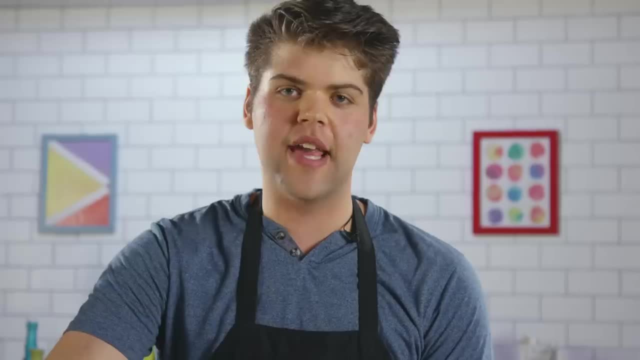 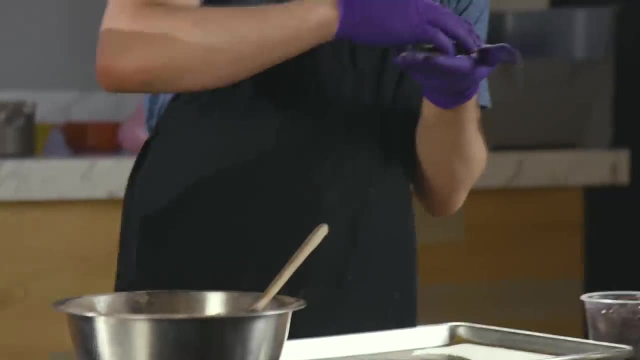 So I'm pushing my cookie dough into the same size cake tin that my cake will be baked in, so that way they're all evenly sized. In order to do some cool decorations on top, I think I might make like some interestingly shaped cookies. 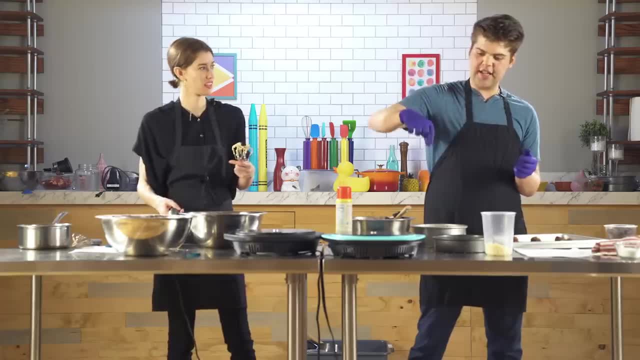 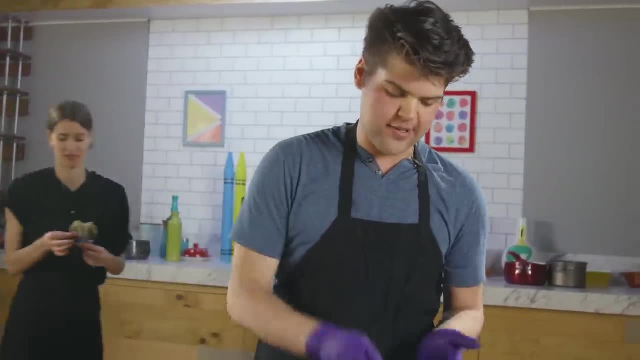 What I want to try to do is make a little like cookie sign that I can like stick in the cake and it'll say Kayla on it. That's so cute If I can somehow spell her name out in white chocolate. Do you want to try this? 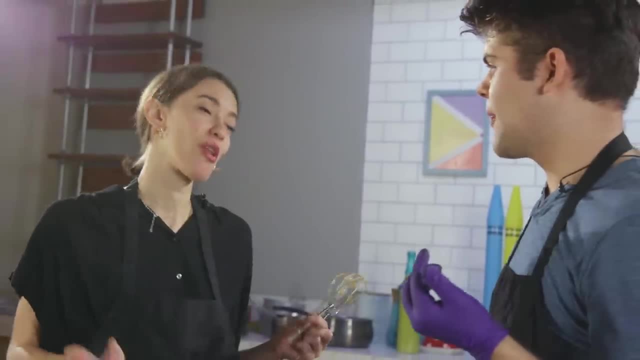 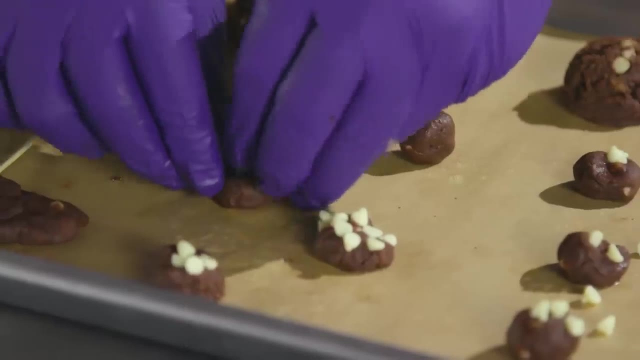 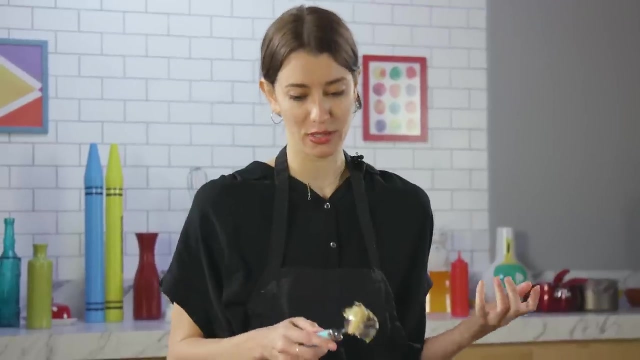 It's good. Wanna try some of this. It's really good. They're both really good. You have more of a chocolate cookie. I do, yes, So that's also gonna be different. Okay, cool, I'm just doing chip on chip. One ice cream scoop equals one cookie, but since I want this to be bigger, maybe three. 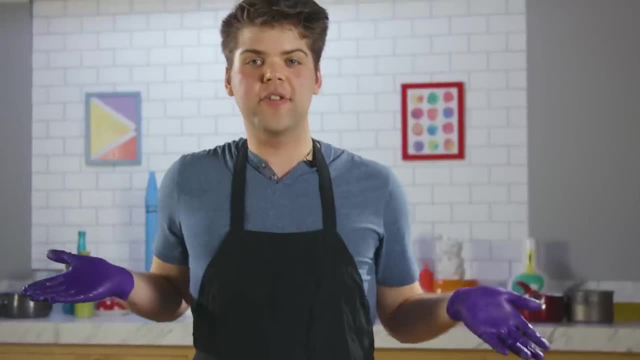 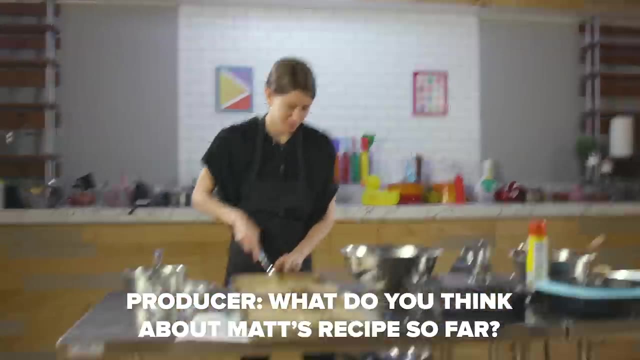 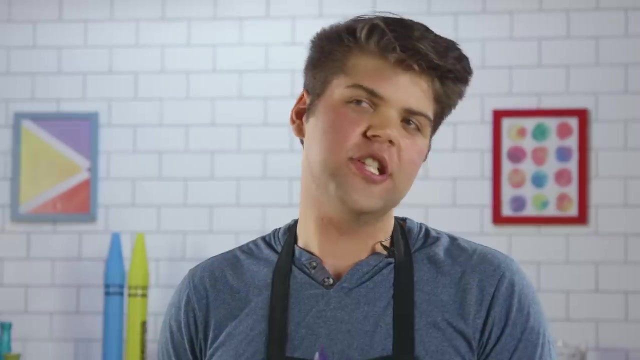 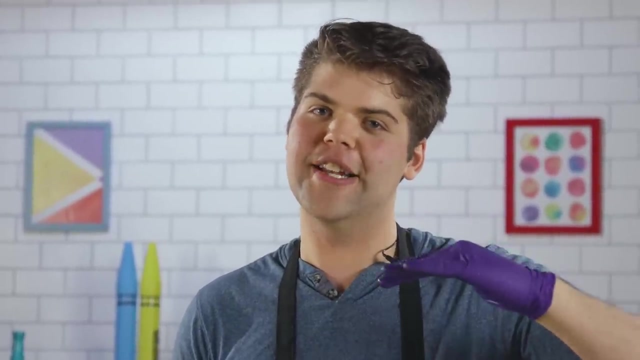 Go big or go home. I'm going into the oven now, Here we go. I mean, so far I feel good. She didn't do exactly what I think Kayla wanted with the cookie. I think maybe Kayla was looking for that chocolate cookie with the white chocolate chips. 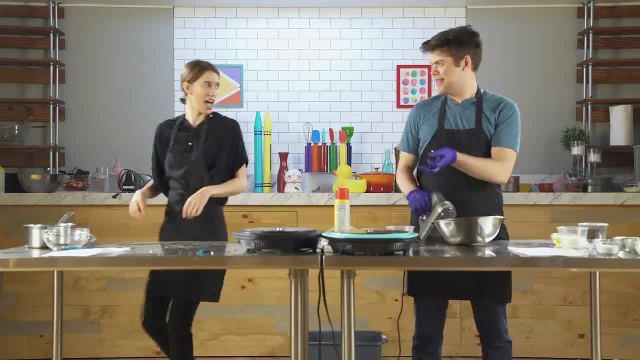 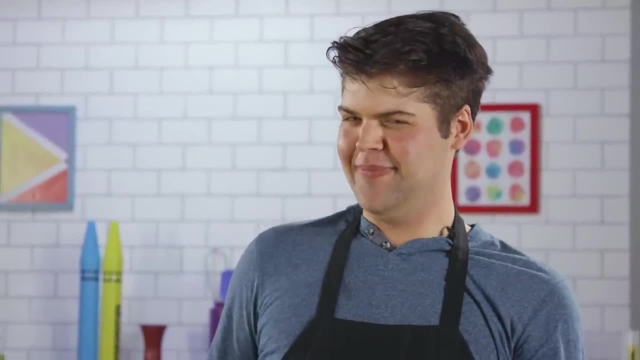 That's what I'm aiming for. While you were gone, they tried to get me to like say some mean things about you. Did you say anything? No, I was like considering, thinking like I could be like bring it on, but that's like so, not my nature. 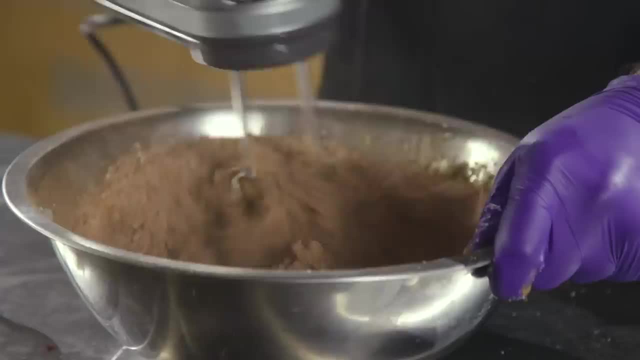 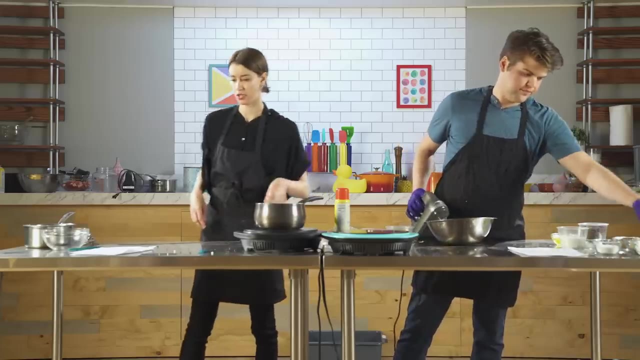 I'm doing the same creaming thing for the cake, just like I did for the cookie. just to help it age a little bit in its being a little more liquidy, I'm gonna add a little bit of oil as well. I am going to. 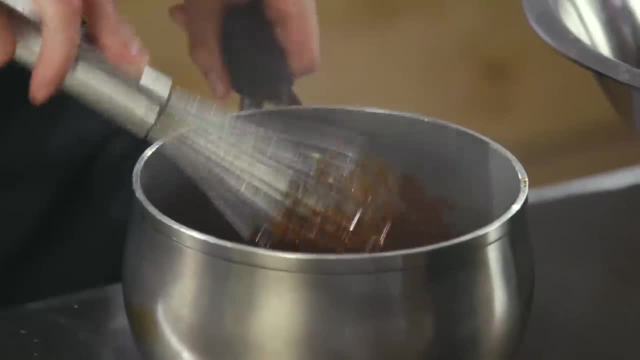 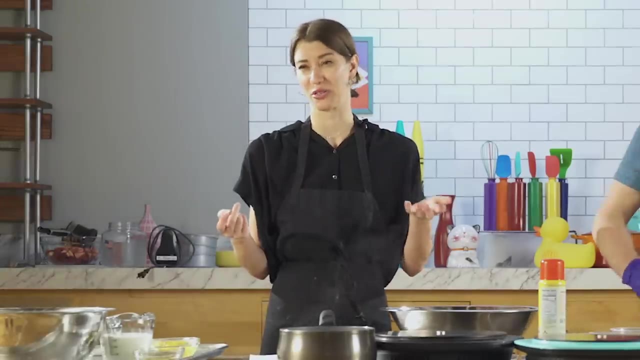 boil water and then add cocoa powder to it as my first step to the cake. The hot water with the cocoa powder is gonna make a more intense flavor than if you just added plain cocoa powder or if you added cocoa powder to cold water. I'm gonna sift the flour, baking soda, sugar and salt. 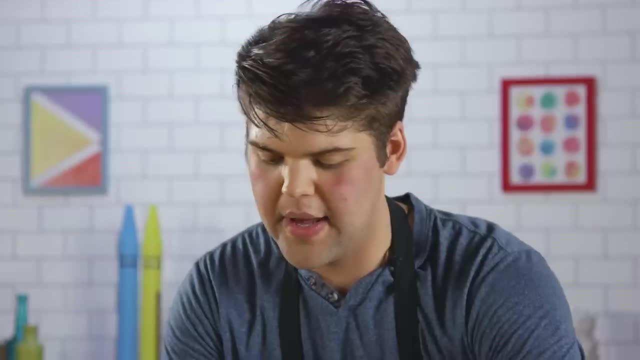 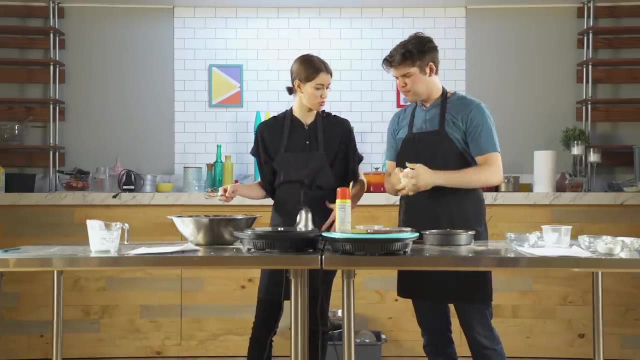 So now adding the cocoa, Now that my cake batter is done, I'm putting them into these cake tins, And so it's actually interesting to see how different our batters are. Yours is much more thick and actually looks more cake-like, whereas mine is like pretty liquidy. 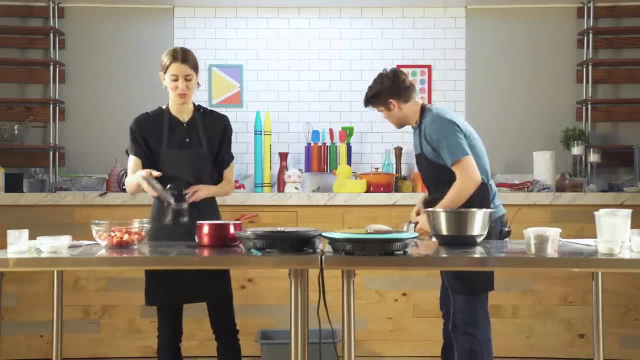 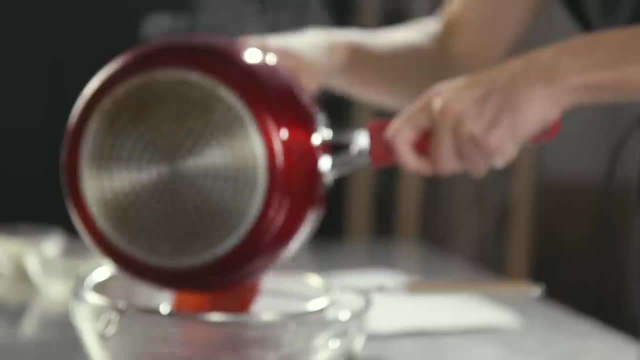 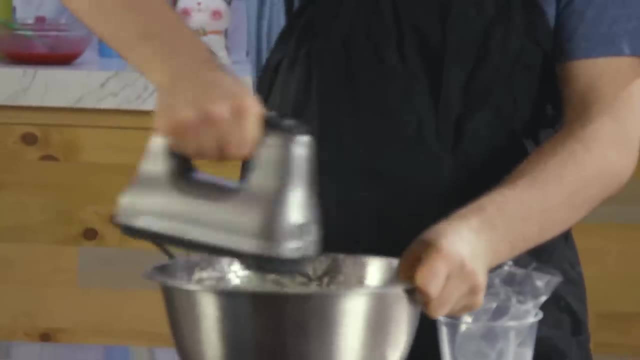 I'm gonna start on my glaze and I'm gonna use a ricer to actually mash the strawberries. I realize this looks kind of gross, but it's just an easy way to get it all kind of pulpy. And now I'm gonna move on to making the strawberry buttercream. I'm not creaming necessarily the butter anymore. 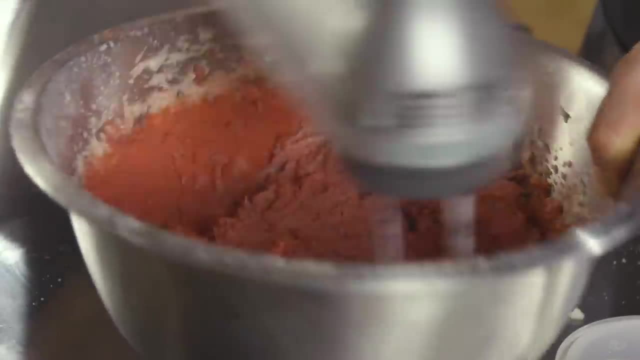 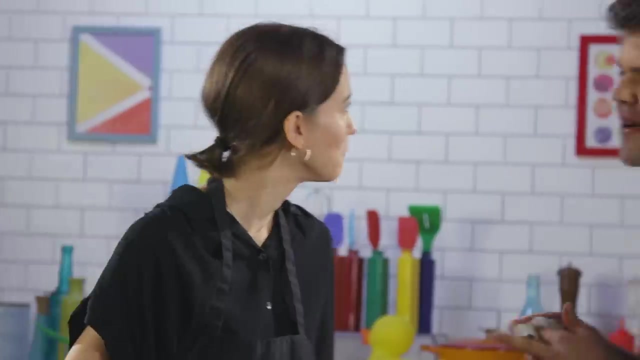 It's more of just like kind of aerating it and then adding the freeze-dried strawberries that I've crushed up And that's gonna give me a really bright pink strawberry frosting. Oh yeah, Almost like strawberry ice cream. Okay, that is so good. 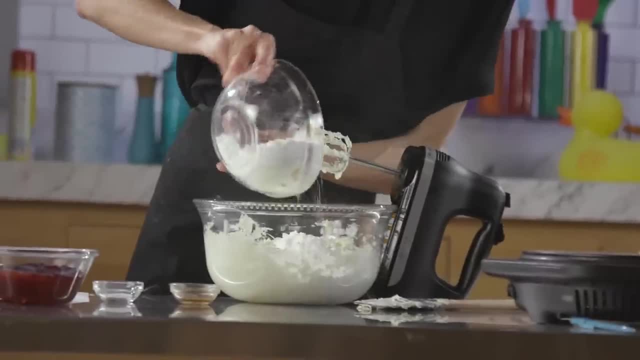 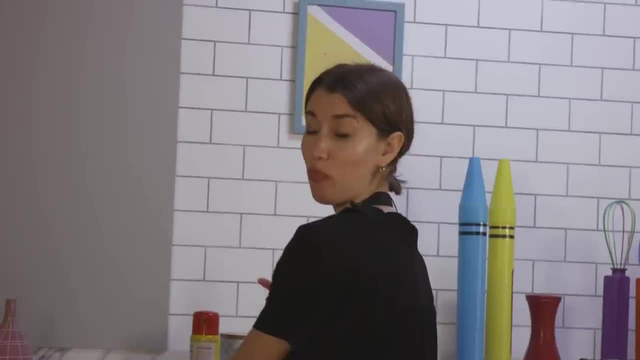 I'm gonna start on my buttercream. I'm going to add powdered sugar, vanilla, again salt, strawberry and raspberry jam. Wow, that's sweet. I think we're at like the easy part that we've all done before, which is like make. 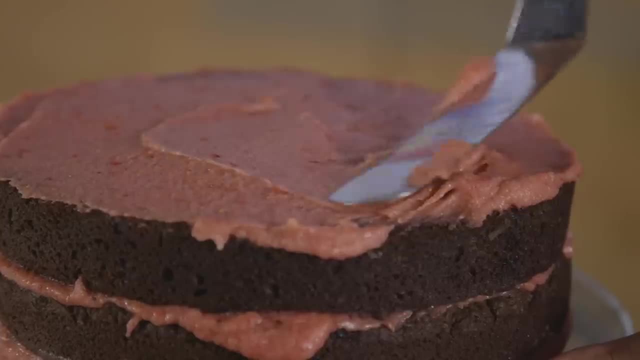 frostings, cakes and cookies. The layering and like the decoration is what's not as confident about. The layering and like the decoration is what's not as confident about I feel really confident flavourwise. I feel really confident flavourwise. 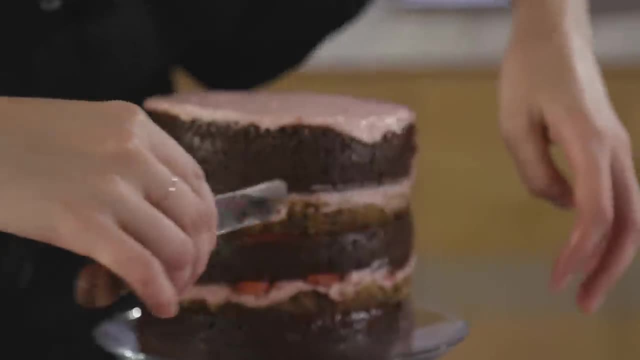 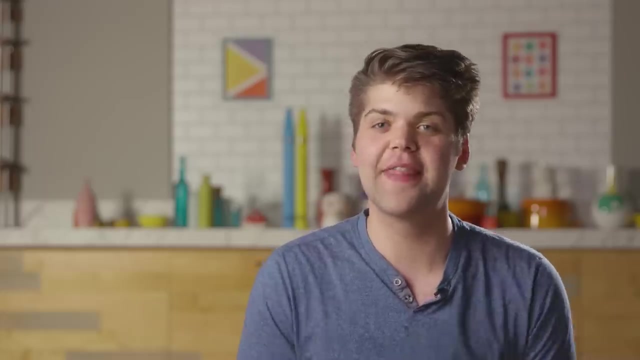 I feel like the decorating What is a nine-year-old like. I don't know. Maybe I'm terrible with kids and I just didn't know it. I'm really excited for Kayla to try my cake. I think it looks so pretty and I have all these little touches upstairs. 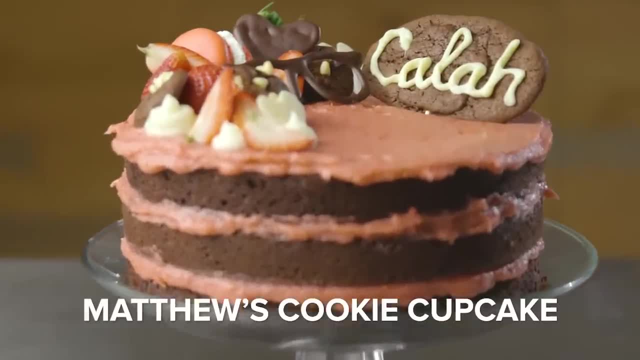 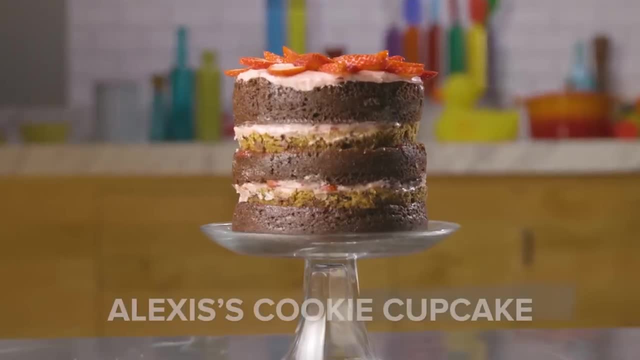 I think she'll really take to her heart. I tasted the cookie and the cake and I like how it tastes. I just hope it's enough to win her vote. I will say that I think my chocolate cake might seal the deal. I will say that I think my chocolate cake might seal the deal. 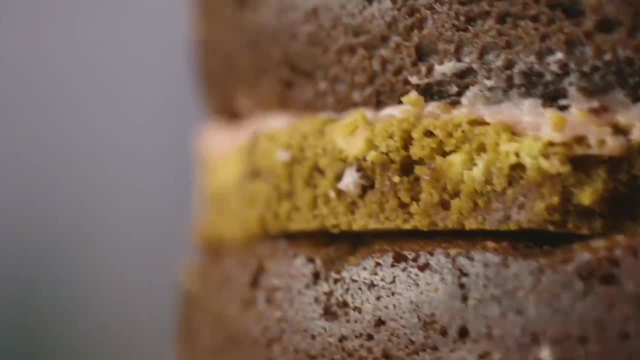 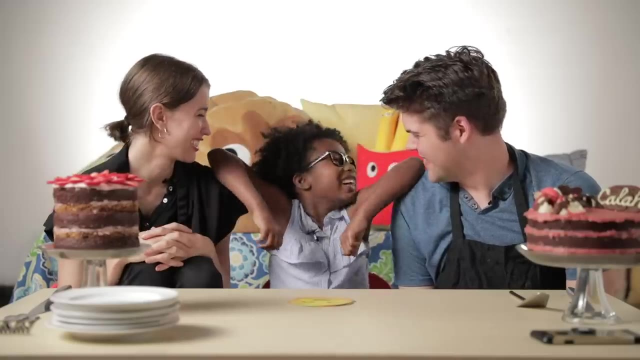 It's so moist and it's so fluffy and I just think when she has a bite of it, it'll be hard. it'll be hard to say no. Okay, you two, what do you got for me? We have our cakes. 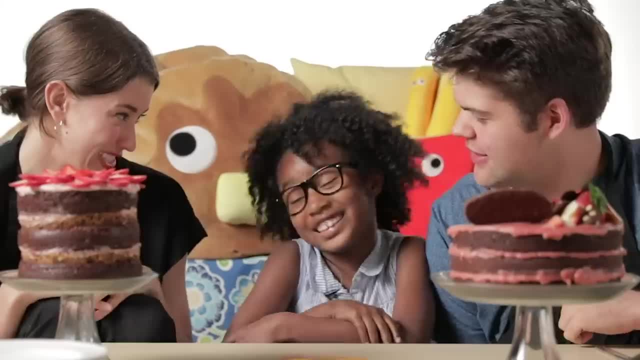 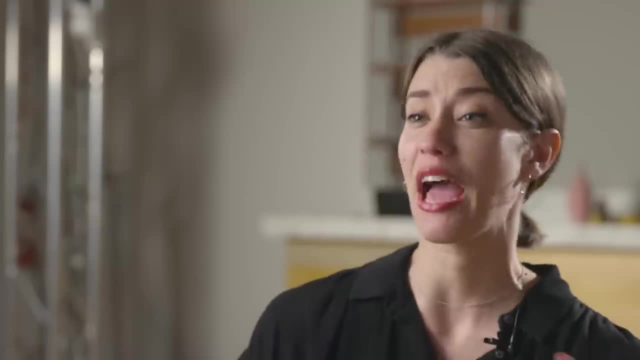 They're a little different from what you drew, but I hope they're good. I hope so. This is really tall. It's like a big, tall tower. Oh gosh, I feel pretty happy with the cake. It looks like what she drew and I think she's gonna like it. 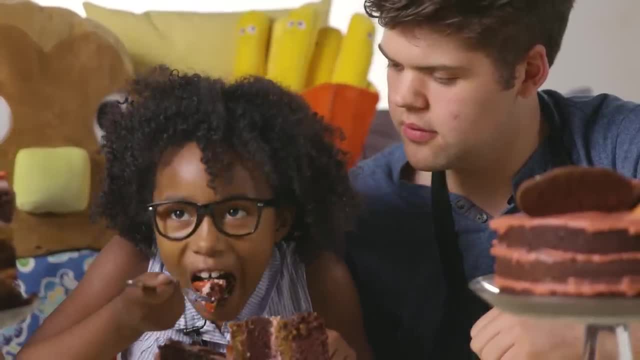 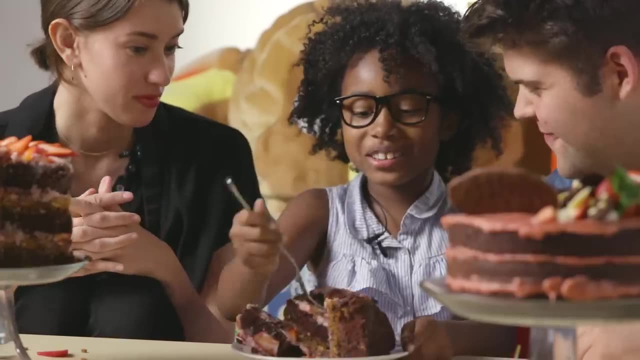 So you know, we've got the chocolatey layers. there's a strawberry glaze, there's the chocolate chip cookies with white and semi-sweet chocolate. Mmm, this is good. Tastes like chocolate with chocolate and it's so moist. 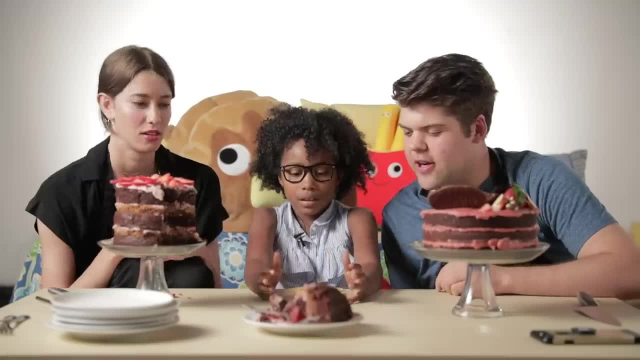 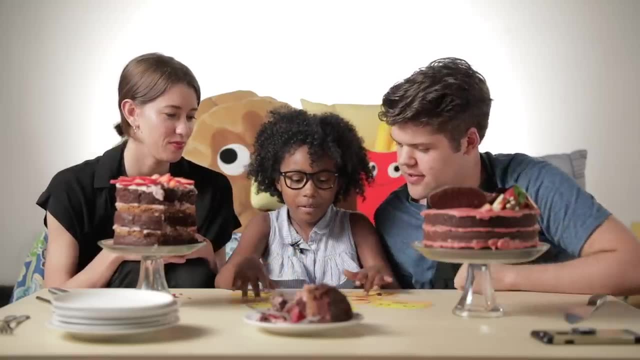 I think she's really into my chocolate cake. So right here we have all these really fun emojis for you. If you had to describe the cake you just tried, which one would you choose? That one, Oh, Thank you. That's such a compliment. 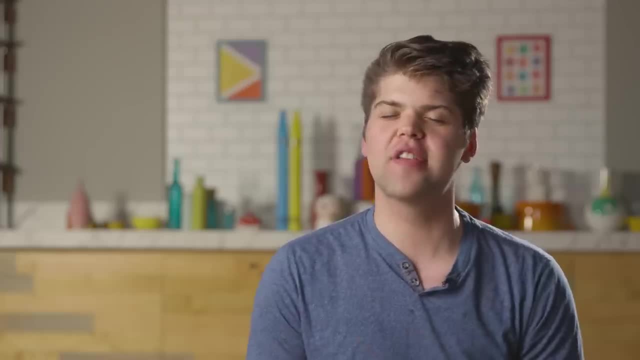 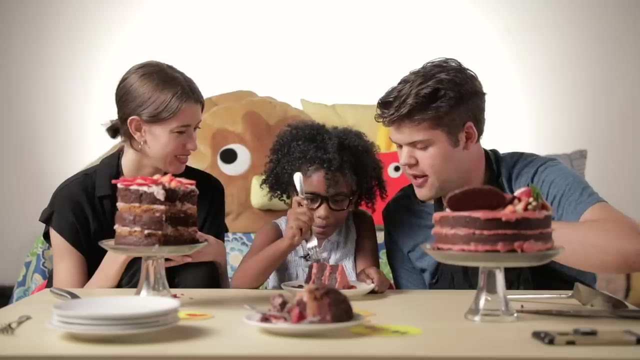 Kayla is about to try my cake and I'm really excited. I know she's gonna love it. I think the cookie with her name on top is really gonna push it over the edge. Here is a simple chocolate cake and then inside there is a strawberry buttercream frosting.